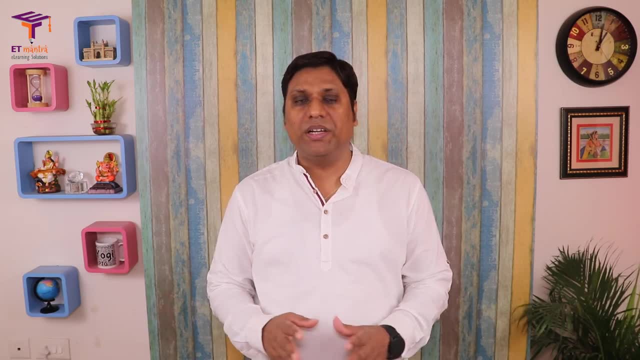 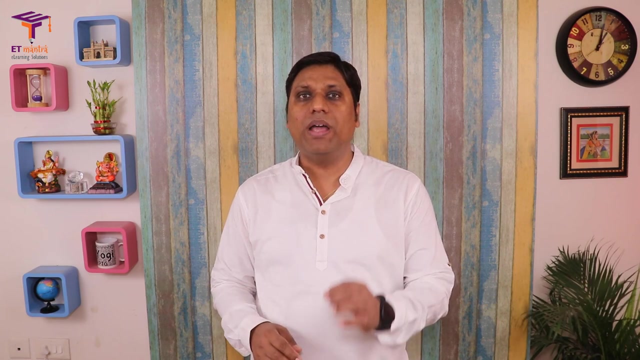 PowerPoint is widely used. It's very popular among the teachers, But do you know that PowerPoint also supports a pen tool? Yes, it has a pen tool. That pen tool allows you to write on your presentations, Not only when you are presenting your slides, but also when you are creating the 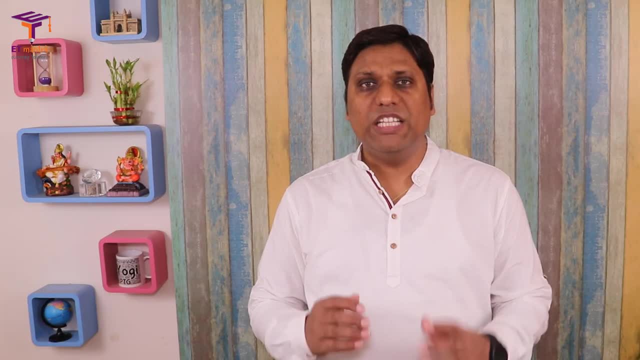 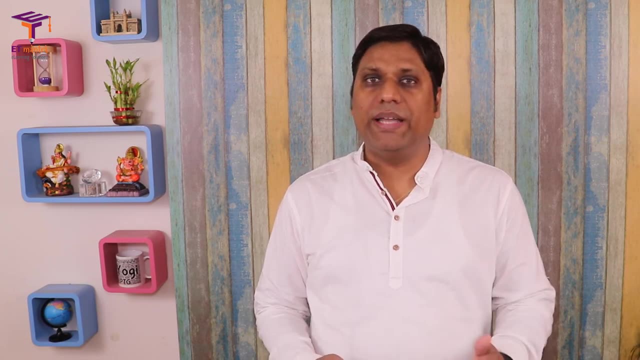 slides You can write with a digital writing hardware. This feature allows to create Khan Academy style videos with the help of PowerPoint itself, And you can also use it as a whiteboard when you are teaching in a classroom or taking a live class, either using Zoom or some other tool. 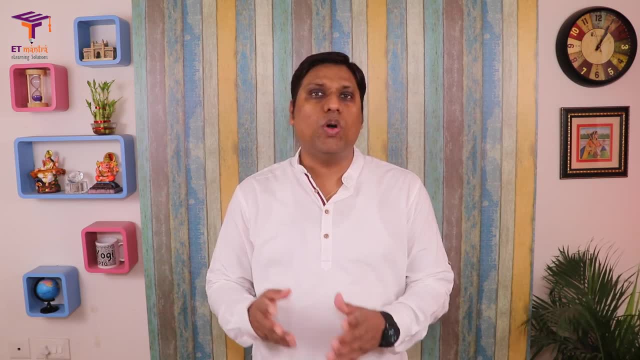 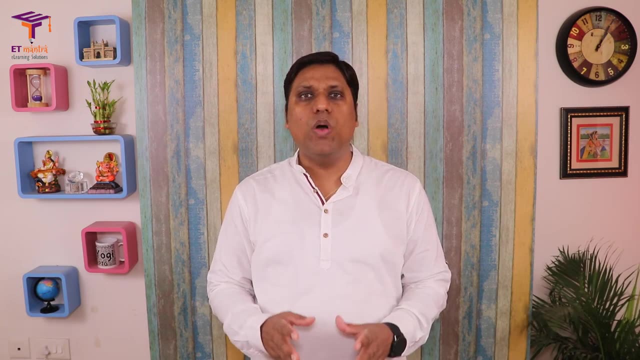 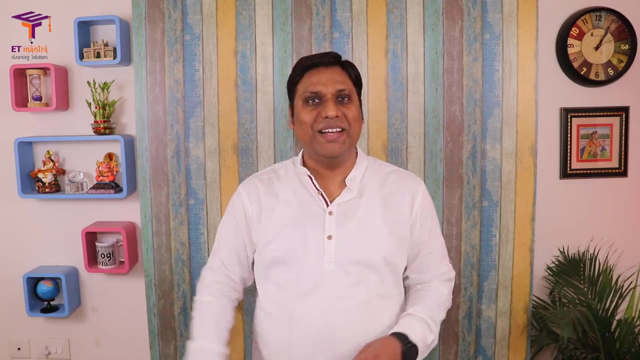 And finally, it depends on a teacher how he or she uses this pen tool. So in this video, I am going to talk everything about this pen tool and how you can annotate PowerPoint slides, either in slideshow mode or when you are editing a PowerPoint. So why wait? Let's start. 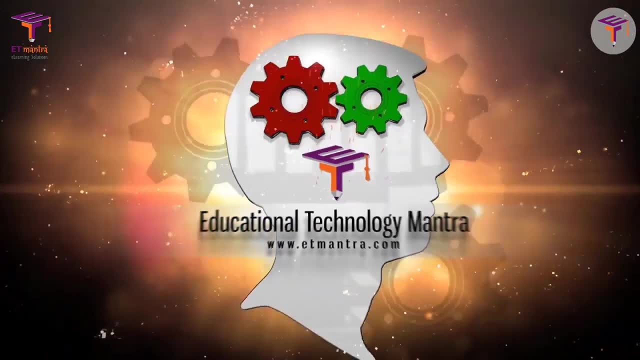 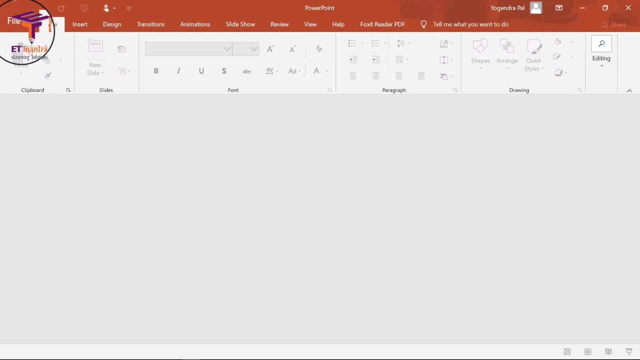 It's very easy to annotate on PowerPoint slides. With the help of annotation on PowerPoint slides, you will be able to create Khan Academy style videos with the help of PowerPoint itself. For that, first of all, you have to open a new PowerPoint, So I'll click on new. 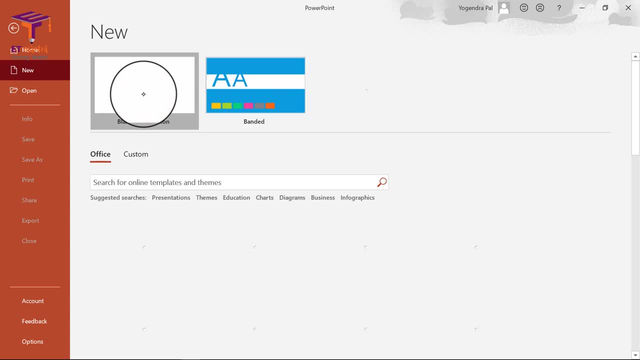 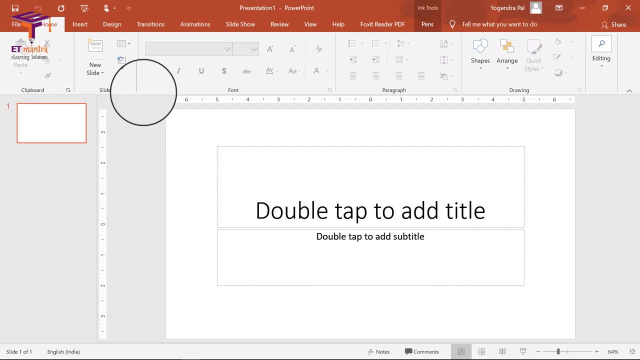 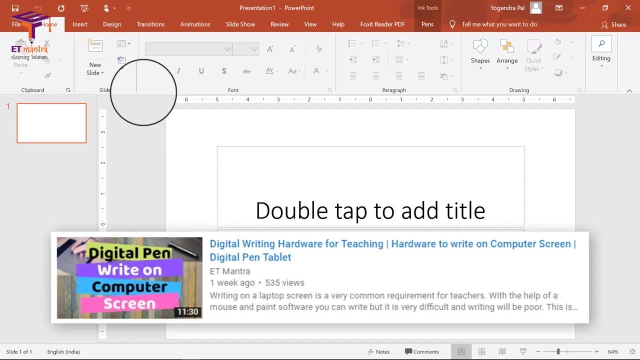 and I'll click on blank presentation. I'm assuming that you want to use PowerPoint as a blank whiteboard or white screen where you want to write everything with the help of some kind of digital writing hardware. I have created a video on digital writing hardware. You can watch the video. The link is given in the description of this video. 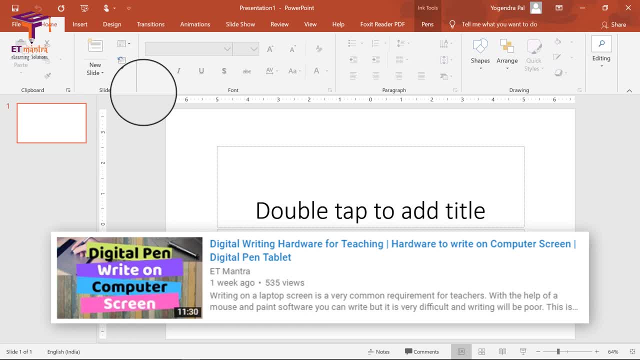 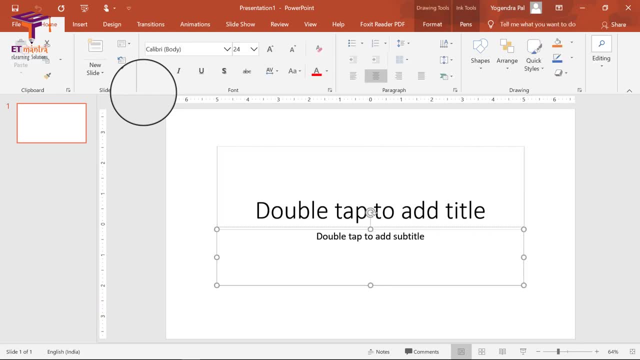 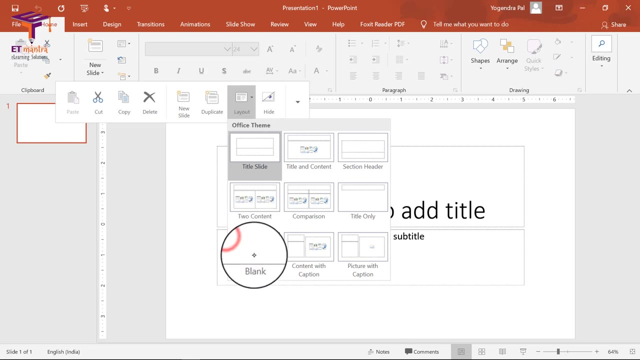 And then you will be able to select a perfect writing option for you. As you can see, there's this option to add title and subtitle. So I don't want that. What will I do for that? I'll select a slide and I will change this layout to blank. See here you will see this blank layout is. 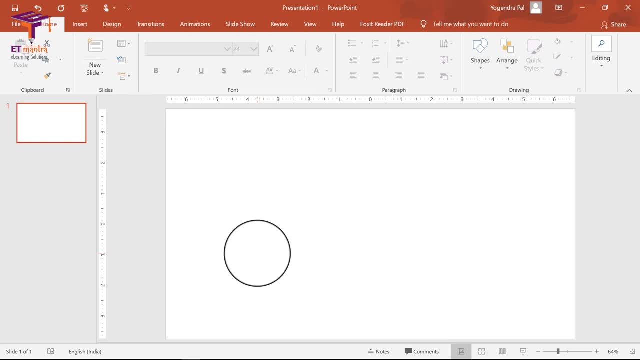 available, I'll click on this blank and now the complete white screen is available with me. Most of the teachers make this mistake by creating a 4 by 3 slide. So don't make a 4 by 3 slide, because it doesn't fit on your mobile devices or television or monitors perfectly For that. 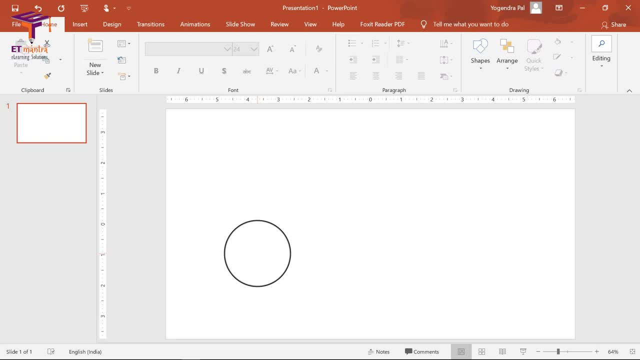 we need 16 by 9 ratio. So in order to create a 16 by 9 slide, you have to go to design. Then here there's a slide size, and then select the wide screen option, not the standard one. Make sure that wide screen is selected. Now I want you to look at the title. 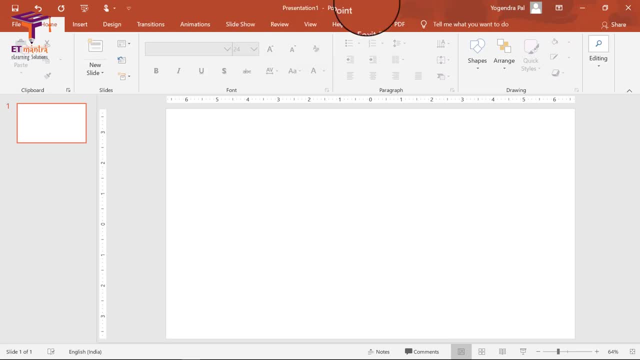 of this presentation. See here on top what is written: Title, name: presentation one PowerPoint. This is written here. Just below that you will see the menu. The menu is view And after that the menu is help. So right now, because there is no pen connected to this laptop. this is why one more option is. 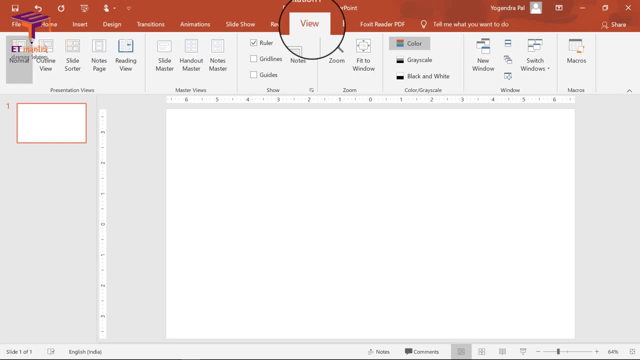 hidden. And what is that For? in order to show that option, I have to connect a digital writing hardware to this laptop. So I'm connecting a hardware. now. See, as soon as I have connected a hardware, you can see a new menu bar available here, which is this: pens. See, the name is ink. 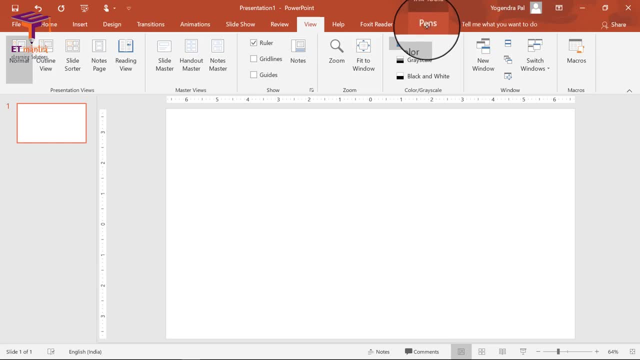 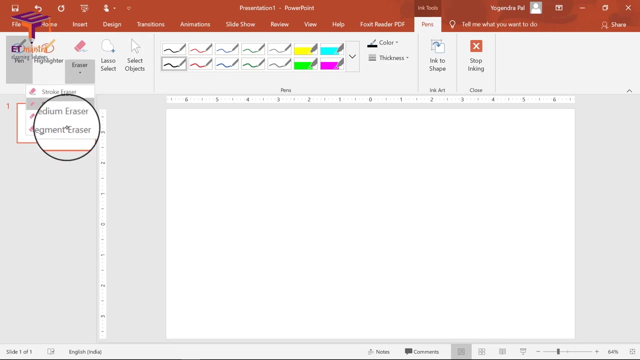 tools and pens is available now. So under this pens menu, under this pens menu you will see a lot of things. It is related to annotating the PowerPoint slides. So first option is pen itself, Then there is highlighter, Then there is eraser and below the eraser you will see a lot of options. So a stroke eraser, a small. 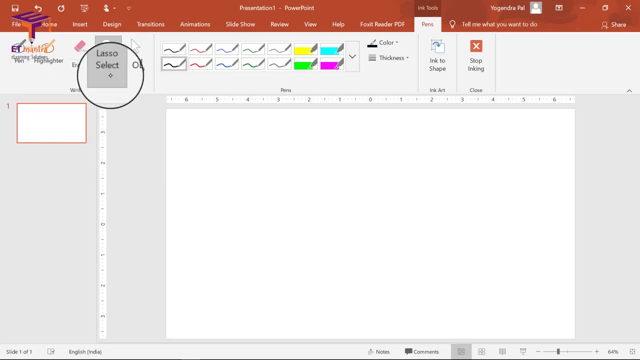 eraser medium or segment eraser- Then there is an option to select something that is less of select. Then, if you want to select objects, you click on this mouse. then you can see these pens. These are the pens from first to last. These 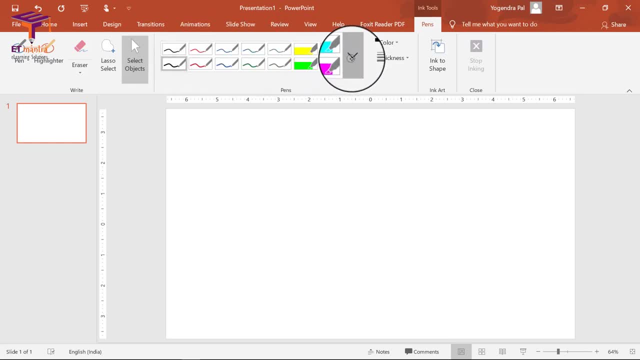 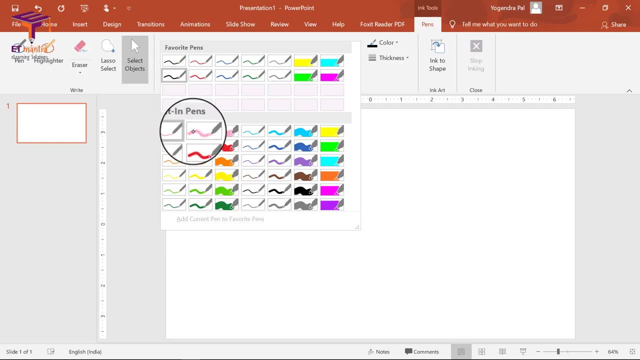 are the pens And these are the highlighters. If you click on this arrow, you will see a lot of options and their width. So, like, for example, this one is pink. So you will see pink. less width means thick, sorry, thin, And here it is thick. Similarly blue: 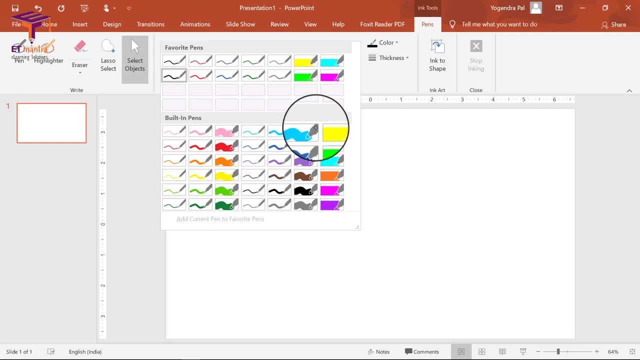 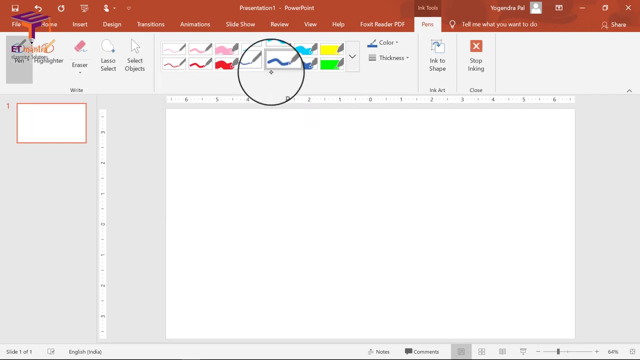 thin and thick. So this way, you have seen a lot of colors here. Similarly, there are so many highlighters Based on your requirement, you can select any pen from here. So, for example, I want to select this dark blue pen with medium width, So I'll click on this and now you can see. 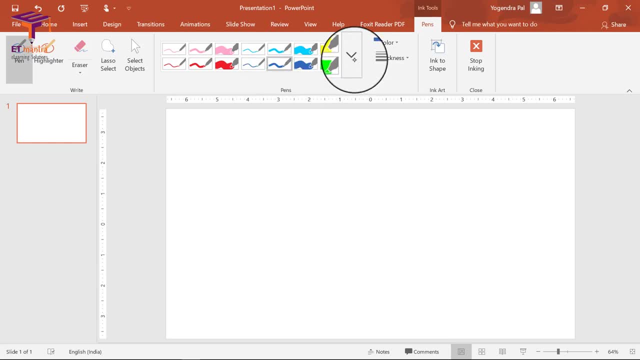 this one is selected. Whenever you want to change the width or color, you simply click here and select the appropriate pen according to your requirement. Then there are colors. You can click on the color. You can select any color based on your requirement. So, for example, if I don't like this blue color, 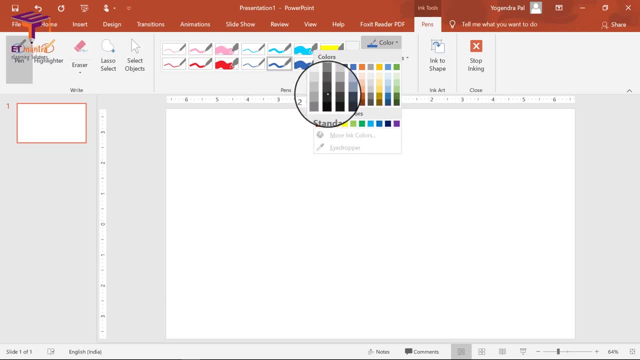 I can select the this, this color, this yellow color. Now you can see this is not selected at all. So the color is this And if you want to select a different thickness, then the readily available options, then you can select a thickness from here. So I'll select a thickness of this. 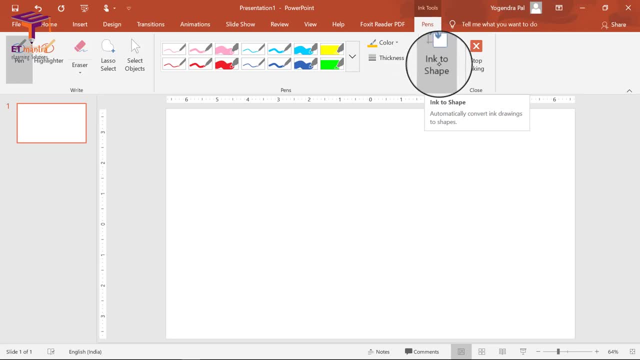 Then there's option to ink to a space. I'll talk about it a little later. And this is when you don't want to write, you'll know. you'll click on this: stop inking. Why they're writing inking? because Microsoft has named it ink option. So once you have a pen and thickness is selected, 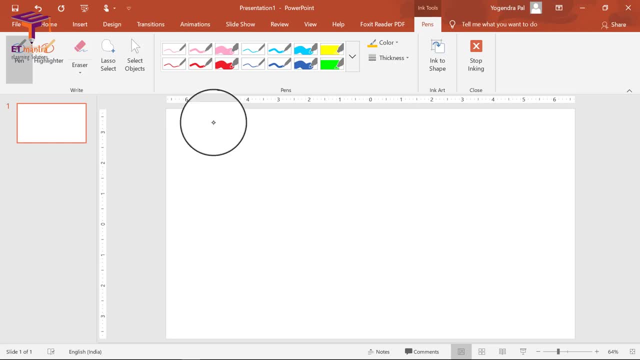 then you can write on this white slide. So I'll start writing. So, as you can see, I can write very easily on this slide and the writing, because I'm writing with pen, the handwriting is good compared to if I write with my mouse. so you can see. 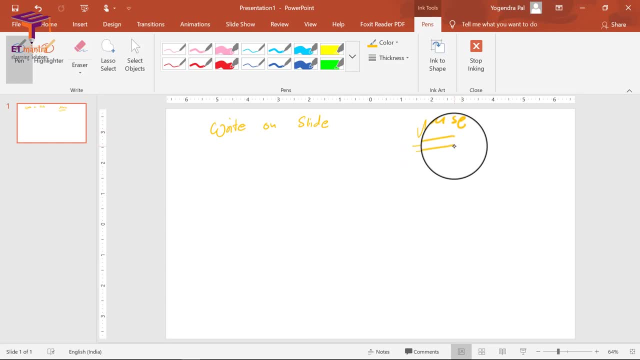 I can write and I am writing very fast. I am NOT writing slowly, so this is the way you can start writing: on slide. as you can see, right now I am NOT presenting it, so it's not slides. I am just writing on the slides, so let me select a better. 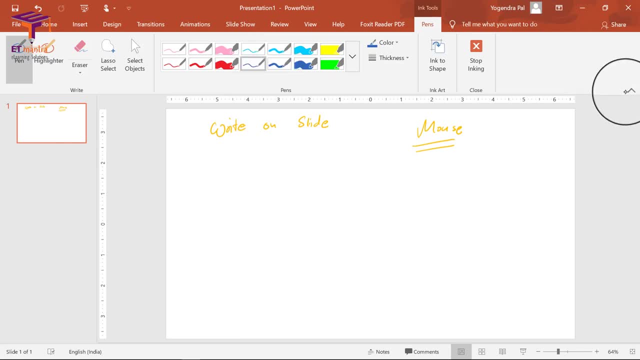 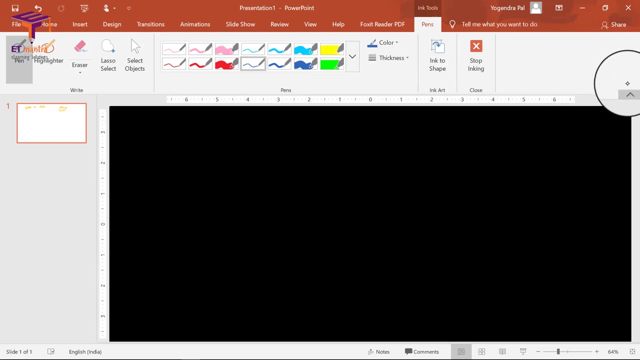 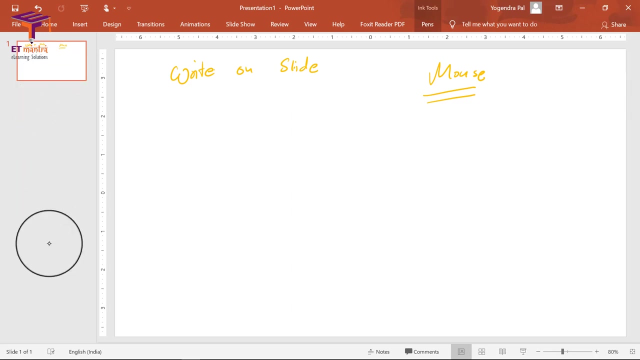 option: better pen which is more visible, then I will hide this ribbon bar. see, this is ribbon bar, so I will hide it. this way I will have more area to write- see, now there's more area- and because I can see the slides here, so I can keep adding new. 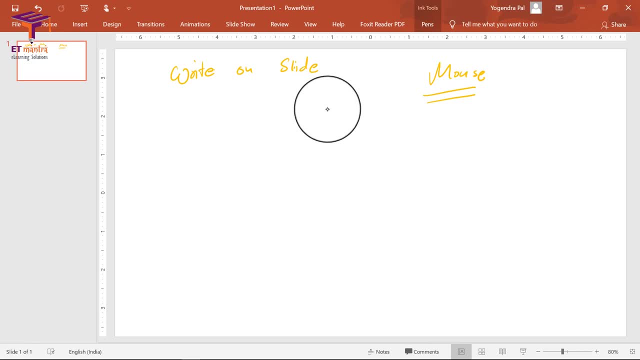 slides here. if I am NOT going to change the pen or its color or thickness, then there is no problem. I can continue, complete my lecture like this, only so let's start writing now. so let's start writing now. so let's start writing now, me, now, right. 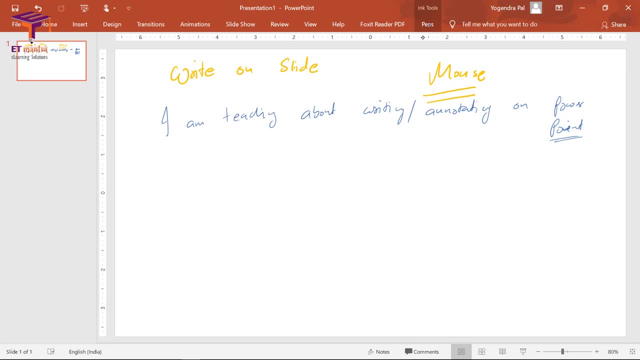 so I don't like this thickness. I will change the thickness. now I will select this color. so this technique was also not good, so I will select a better thickness, like this, and now I can start writing: see, like this, like this, so you can draw whatever you want. so like this. 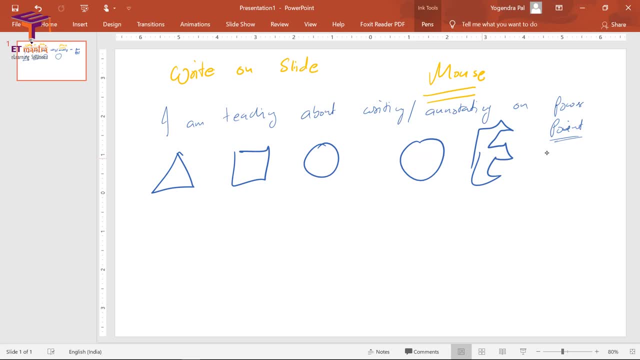 you write whatever you want now, wherever. whenever you want to delete it, you again go to Pen menu and select our eraser. so this way you will be able to get it. so, as you can see, this Erase Erascary is erasing the strokes, any strokes. it кар 니 иг USА. 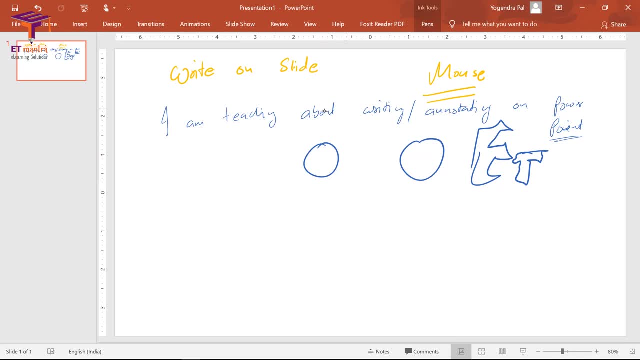 any strokes, which it is very interesting for me. so under goes Eraser. I am gonna start out with this one打ью. it is touching. for example, you can see here this: u and t are one stroke. so if i select t, the u will also go. see, u is gone. similarly, if you check all the options of eraser, there are 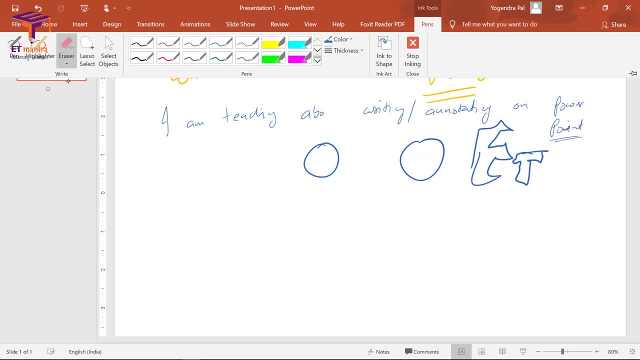 other erasers like this. a small eraser is there, so this small eraser will actually work like a eraser. see, it will not erase complete stroke, but it will erase only the portion from where you are moving it right. similarly, there are these other options also. now you can try them then. 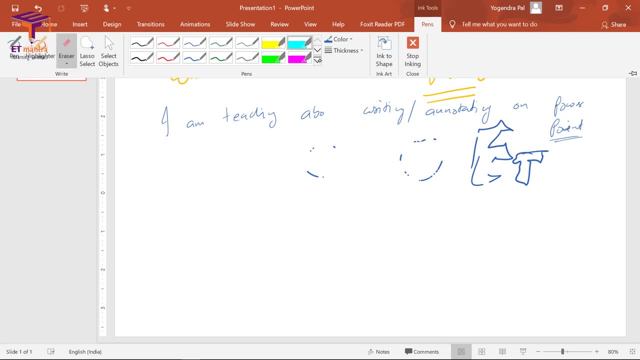 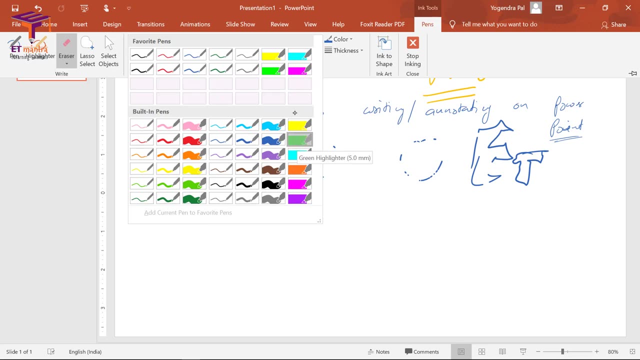 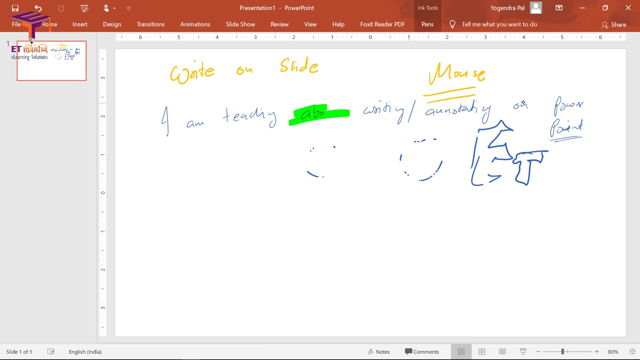 there is this highlighter. highlighters are available here also see these. this last two columns are highlighter, so let me select this highlighter and i can now highlight, so you can highlight very easily with the help of pen itself. let me now see. i think this is not highlighter, this is pen. sorry, the last column is highlighter. this is the. 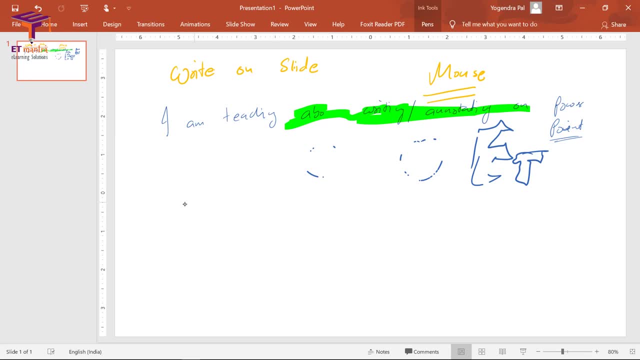 pen with the very thick option. so this is how you can write on the slides. whenever you want to add a new slide, simply click on this option and add a new slide. click on this new slide. the new slide will be added, and then you can start writing here also. 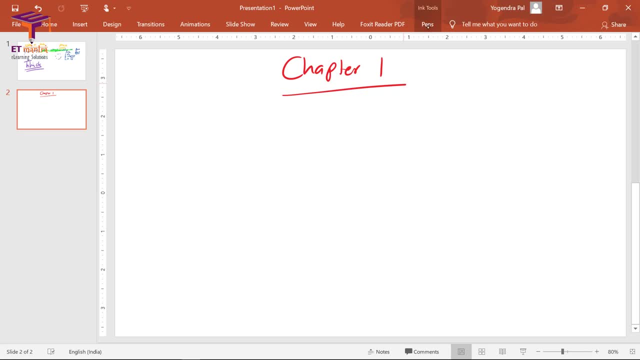 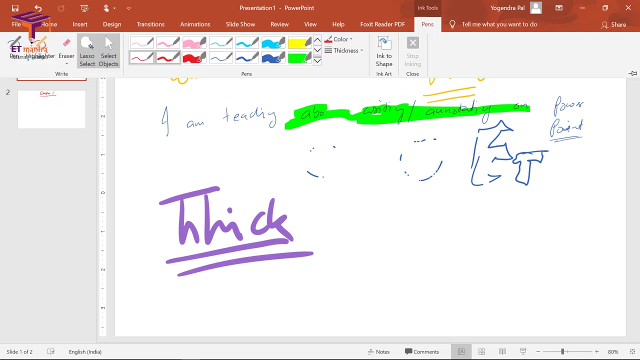 like this. let's see other options in this menu. this is lasso select. so what does it do actually? so you can select a lot of area, a lot of component from the screen just by clicking on it. for example, i am going to this first slide and now i will select this lasso select, and now i will select this teaching and on. only so i will. 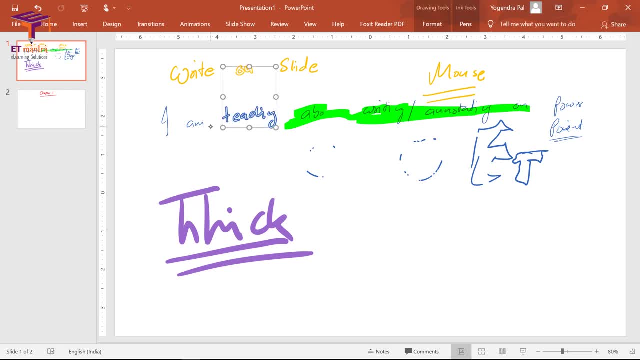 move my pen like this: so this is now selected and then I can delete it by right-clicking on it or I can move it around the screen. so let me move it. now. see, this is how I can move these options, or I can delete it also, I can delete it. so if you want to select more than 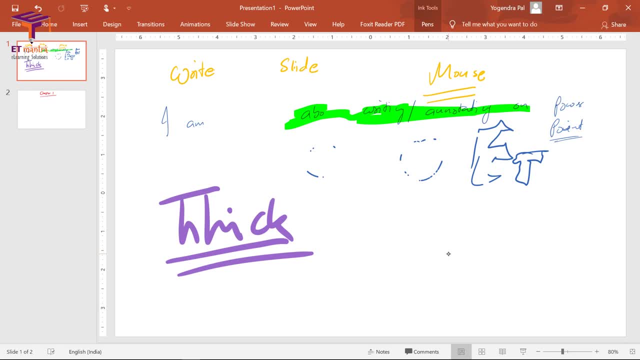 one component, or if you want to choose some element by choice, then lasso select is the correct option. then this is to select object: simply click here and with the help of this you will be able to select the complete objects. so complete object is now selected and I can. 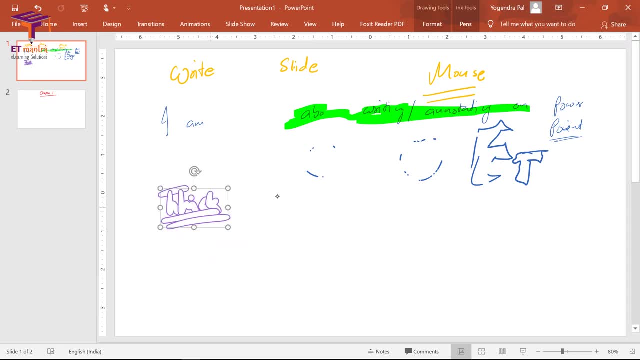 resize it, I can move it, I can rotate it, so you can do a lot of things with the help of this select option. then now let's come to this ink to shape. it is a very good feature. I want to demonstrate this to you. so let me go to another slide and let's select this: 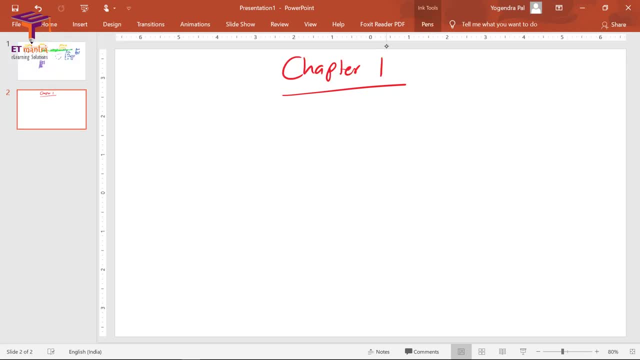 ink to shape option, so ink. you understand, Microsoft has given the term ink when you are using pen on its operating system. so because now ink to shape is selected. so this way, if I want to make a triangle, I will make a triangle like this and it will be a perfect triangle. 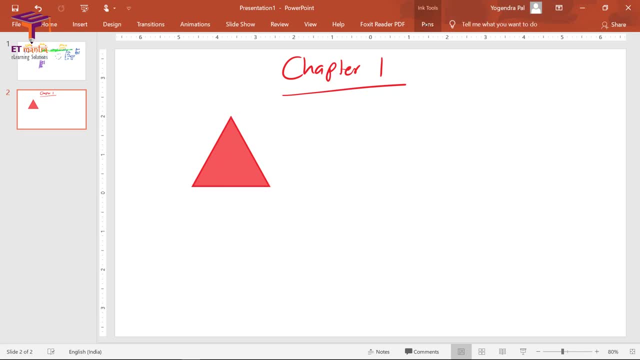 so it will become a perfect triangle. similarly, you can create rectangles, pentagon, circles with this, the help of this ink to shape option. so this is how you create your slides once your teaching is complete. so you start creating multiple slides once your teaching is done, you can. 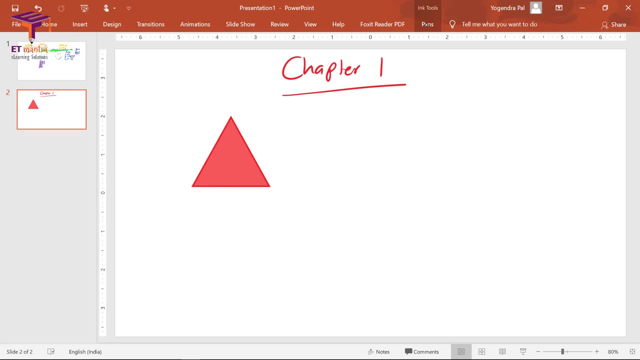 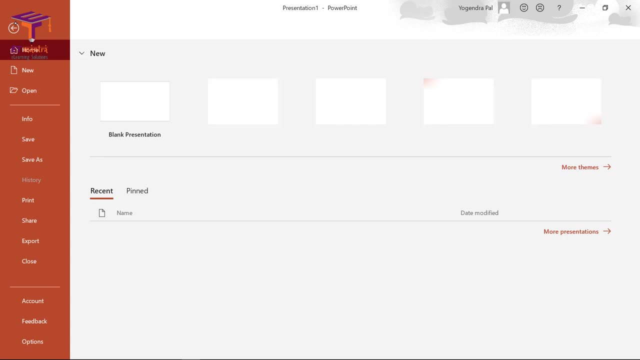 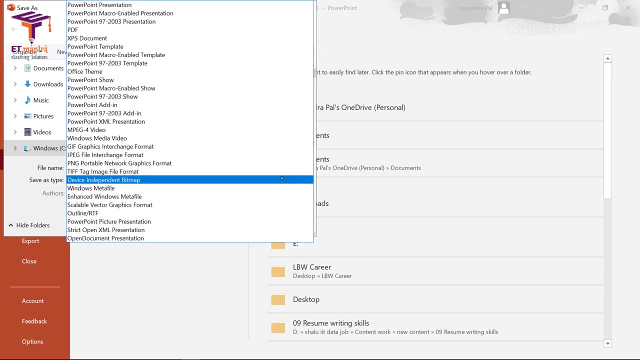 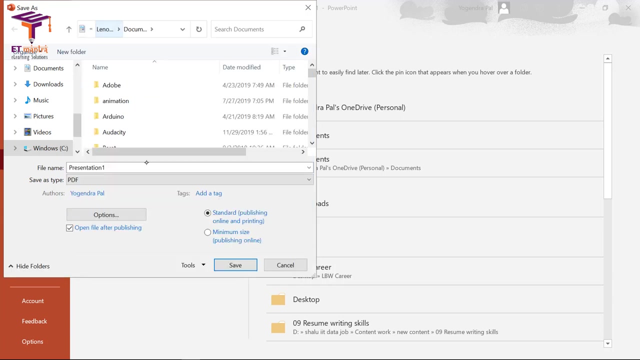 share this file with your students by saving it into PDF or PPTX or PowerPoint slides. so so, by simply clicking on this file and then save as, just make sure that here in this option, you are selecting the PDF option, so you the PDF option is available here, I e select the PDF and then I will give it a name. I am 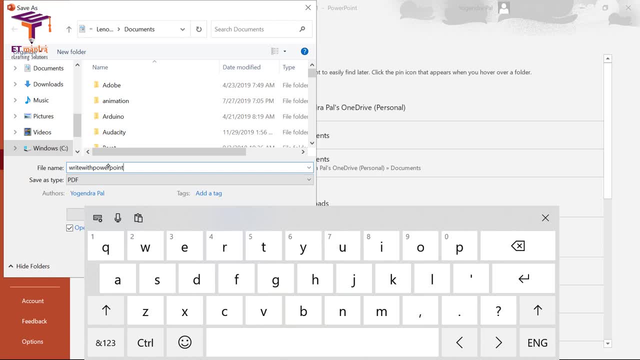 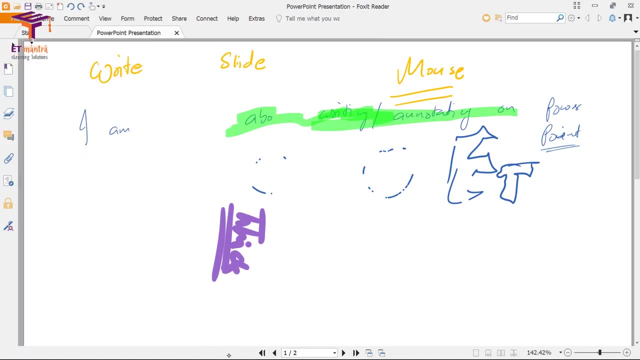 giving this name so that it's easy for me to share it with you, and now I'll save it. so it is now saved in PDF format. so this is open in Foxit reader. you can see there are two pages and I am on first page right now. I can go to second page and see this is the second page. I am on first page as well, so I can go to question fast. so when I click on next, I have to help. description: I can see there is a the post, or I'm not, depth definition. anyways, let me just only completely guess at a topic and then I'm gonna ask- I'm so that it the feature name for last page, because I none. 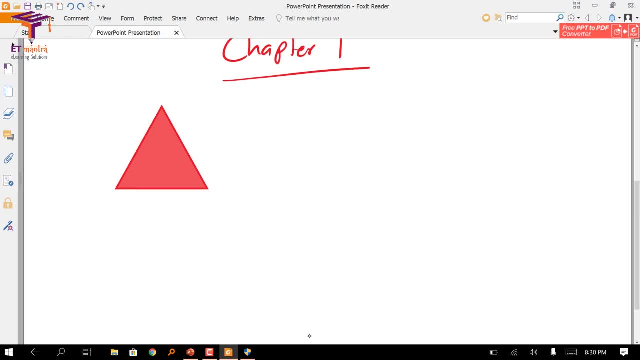 the second page, you can see the quality of this pdf is also good and you can easily share it with your students. so not only your video will be created. if you are using a screen recorder while you are teaching with the help of powerpoint by annotating it, your video will be created as. 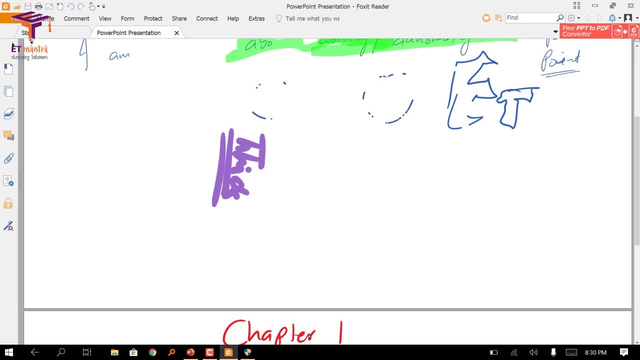 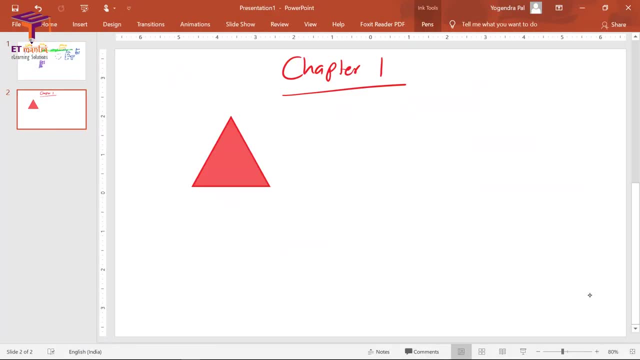 well, as you can later send this file to your students in pdf format also. let's now see what if you want to write while you are presenting your slides? so right now, if you want to create a video with this setting, you have to select only the slide area. this means your recorder screen. 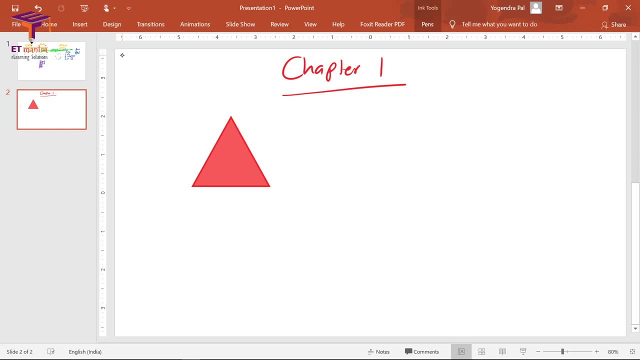 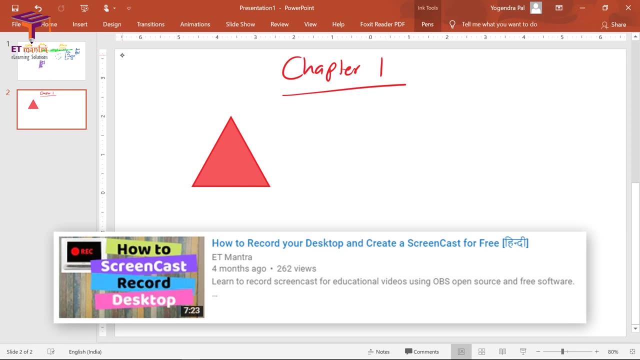 recorder should have the facility to select some portion of your display. that is available in most of the recorders right now. i use camtasia. it is available in that. i use obs. in that also, i can do that. but let us say you want to utilize complete screen, so i can do that. 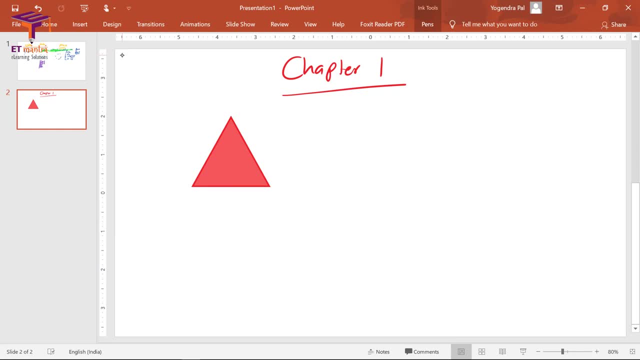 because you also want to record your video in high definition or full HD. so let's now present the slide for that. I will create the desired slides first here. so I will create a lot of blank slides because later while teaching using the slide. so I don't want to come back to this. 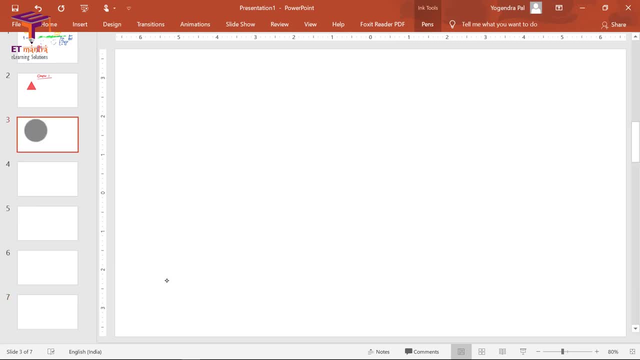 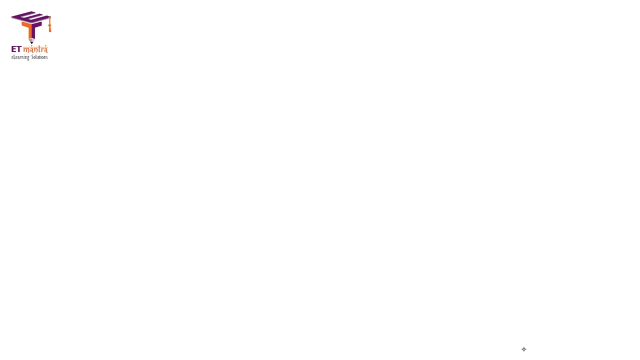 slide. okay, so I will now present it to full screen. basically, I am going to create a slide, so now you can see that I have started the slideshow and this is why you can see the complete white slide is in full screen now. if I bring my pen, you can see this red dot here. okay, this is actually. 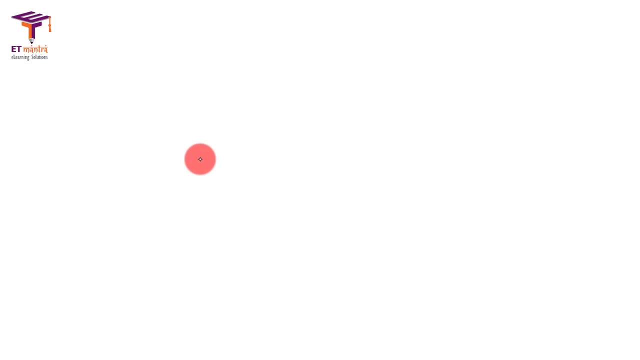 where my pen is. I am hovering my pen over this laptop right now. I will come to the bottom left section of this slide with the help of my pen, and there you will see a lot of options. one is the search option, then there is some other option, then there is this ink option and there 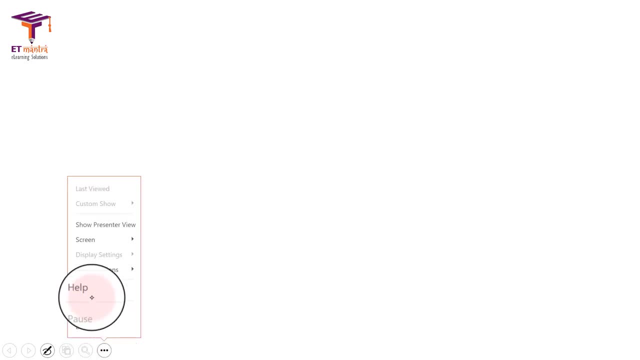 are some other options also, for example, eraser arrow option screen or screens show, presenter view screen and many other options are available here. I need I need to worry about this pen option only, so I'll click on this. click means I will tap with my pen over it and here you will see laser. 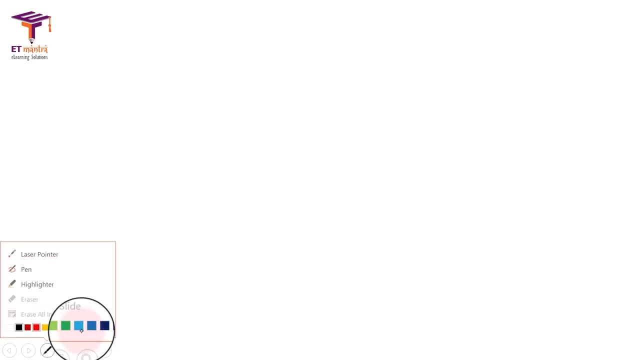 pointer, pen highlighter- then you can select different, different color options also from here. I I'll check if I can change the width of the pen or not. so no, the width of the pen cannot be changed, so I will select a pen. here the red color is selected, I will select this dark red and then I 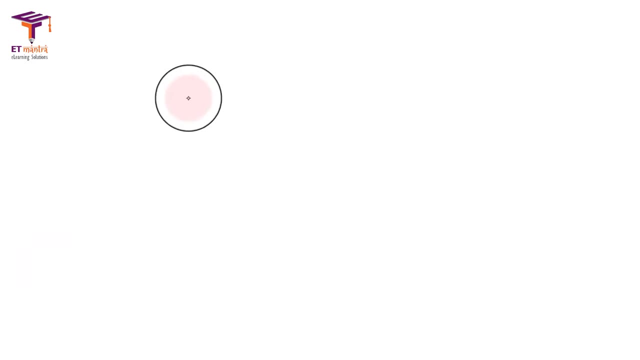 will select the pen. so now I have pen in dark red color with me and now I can start a scribbling on PowerPoint slides. so this is how you can teach. you need to spend some amount of time in order to become habitual of software options and hardware. 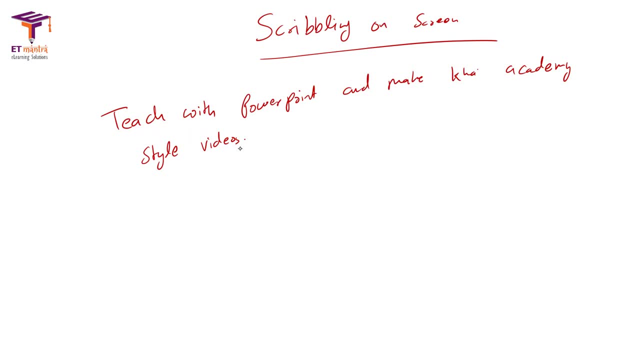 pen. so once you think that you have taught everything for the slide, then you can start. then you can simply go to another slide with your mouse or with the touch screen option. then this is another slide. so I will write slide 4 here. if I want to teach something, for example this, I can do: 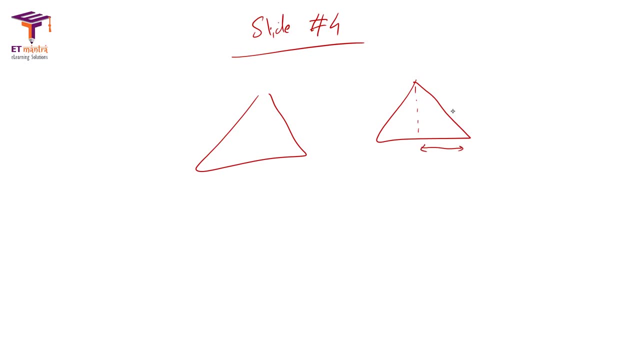 this also ok, so you can teach math, science, biology, physics, chemistry with the help of this, with the PowerPoint and writing on it with the pen. then I'll go to another slide and here also, let's change the color, so it's not like that you can't. 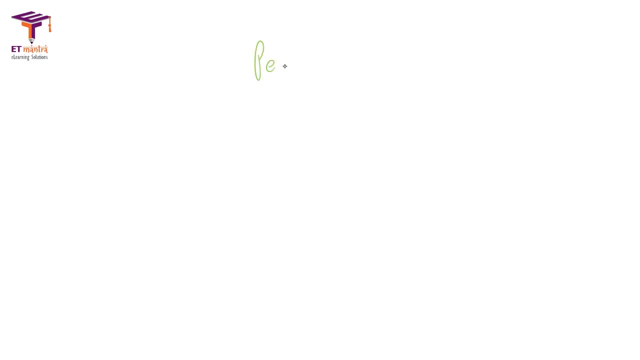 change the color of pen. you can always change the color of the pen by going to this bottom left corner and selecting a different color. so right now there is this blacker. let's now see these options also, because they are also required many times. for example, this less laser pointer is required many times when you 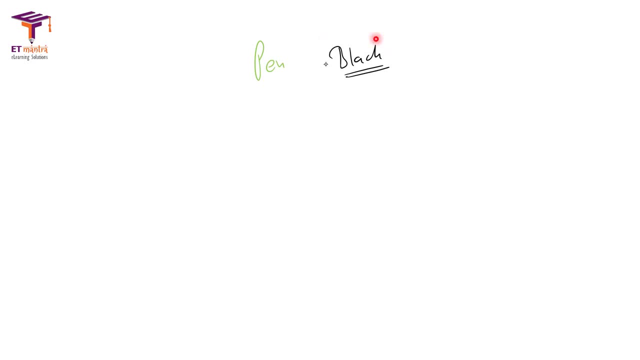 are explaining things. okay. so right now, like I am moving it like this and then here, so you want to display pointer options. sometimes, similarly, there are other options also, like this: eraser is available and highlighter is also available, so let me just highlight this. so this is how you can highlight and 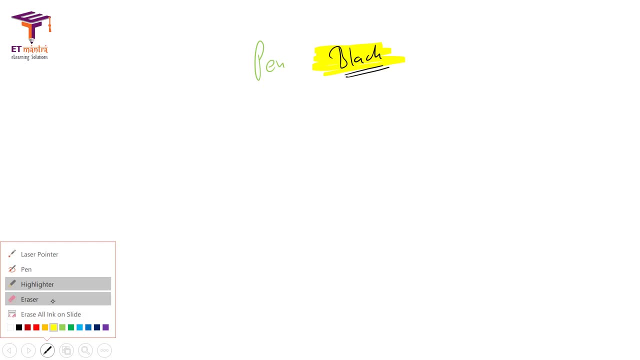 you can also change the color of the pen by going to this bottom left corner. and let's now see this: it is. it is option. I will erase this option. okay, now there is an another option: erase all ink on slide. so you can by clicking on this, you can. 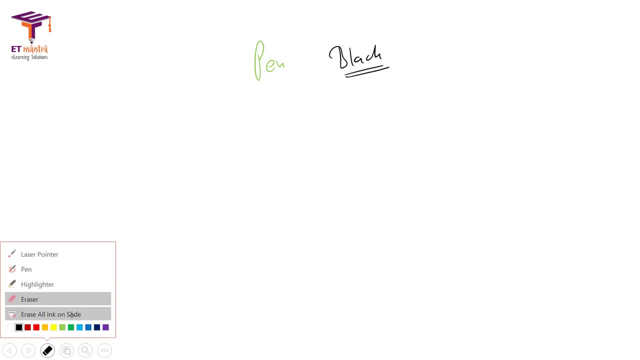 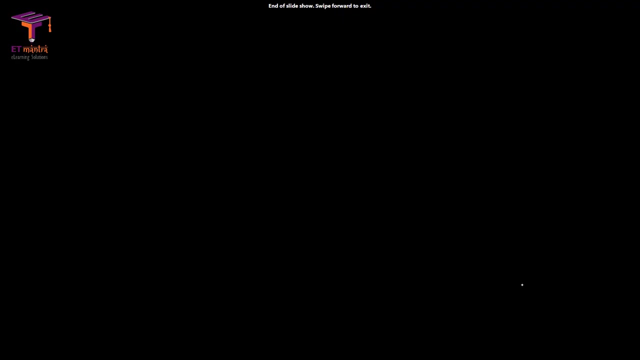 erase everything whatever you have written on the slide till now. so these were the options when you are presenting a slide. let's now go to another slide, let's again go to another slide and let's now end the presentation. so this is how you can change the color of the pen, and you can also change the color of the pen by going to this bottom left corner and 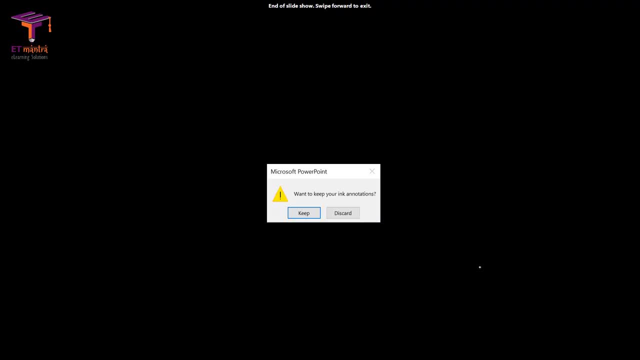 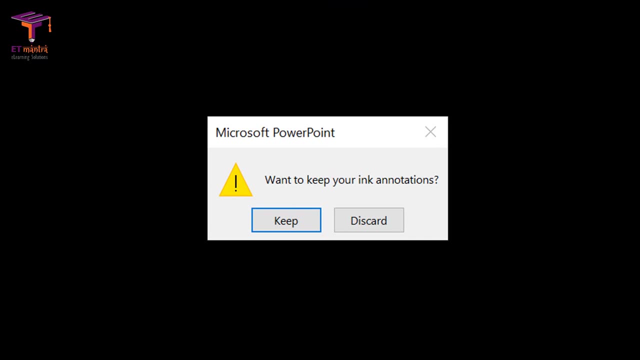 the presentation is now end. when I will end the slideshow, it will give me this option. this is very important. it's asking you if you want to keep the ink annotations or not. if you click on discard, all the annotations that you have made during your slideshow, they will be discarded. but because I want to, 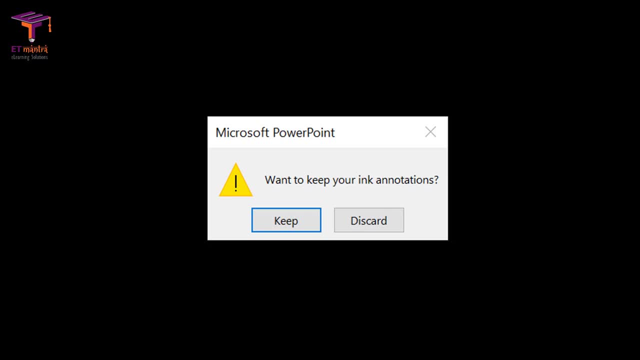 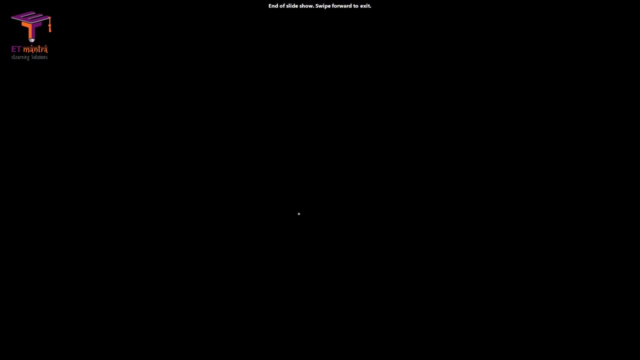 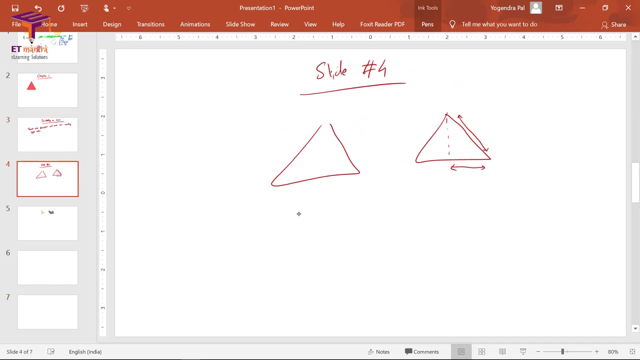 give to my students as it is. if you are making a Khan Academy style video, you have to give the notes as it is. is then what you will do? you will click on this keep, then slide will end and now you can see all the scrabbling that you have done during teaching on slideshow is available on the slides. 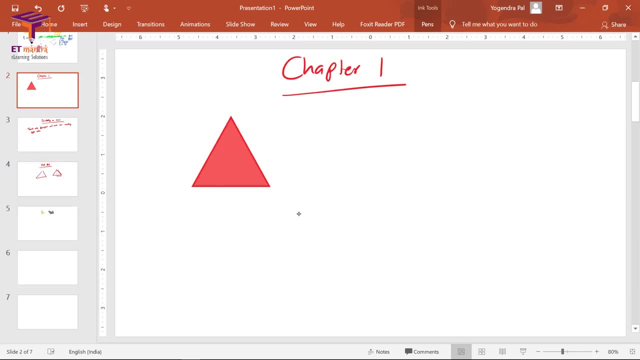 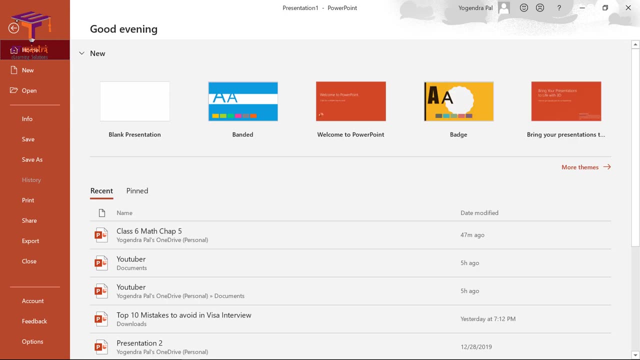 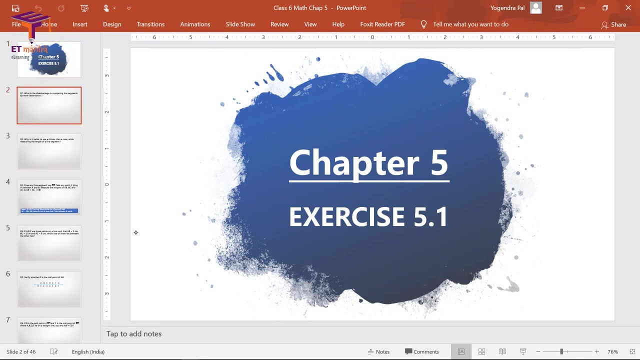 see. now you can share it with your students by saving it in pdf format. if you have a presentation, pre-prepared presentation, for example, i have this presentation. let me now open it. so this presentation has text written on it and sometimes there are notes. also like this: sometimes there are. 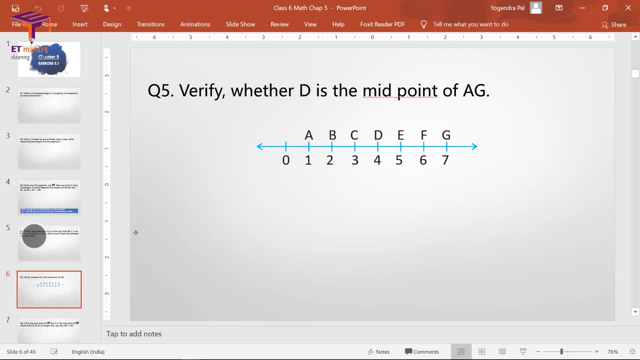 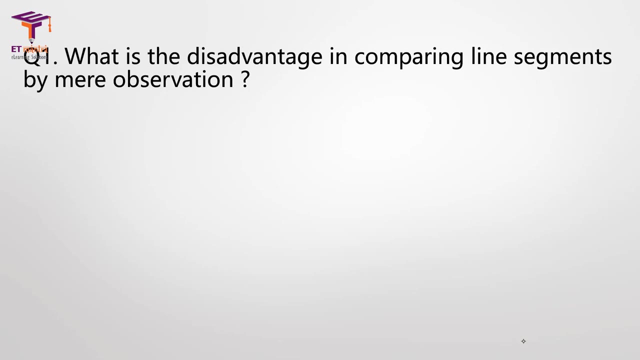 some graphics elements available. okay, so if these options are available, even in this case you can draw or you can annotate on the slides. let me now present it in a slideshow mode so, as you can see, the text is already there. so it is also a use case when you want to write the question in advance. 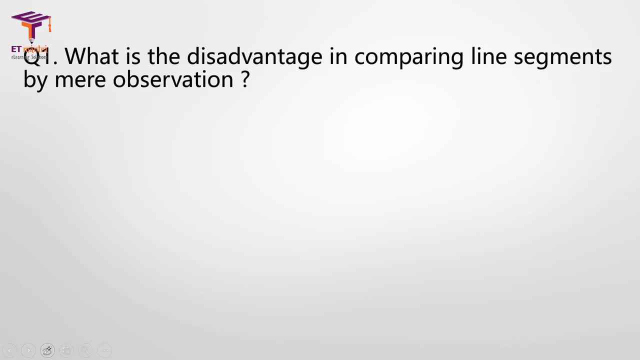 on slides and then just present it with the help of pen. so you will click on this pen and now you can start writing, start highlighting, for example, this: you can draw, you can highlight the text like this. so you can do a lot of things with the help of the options available in the powerpoint, whenever 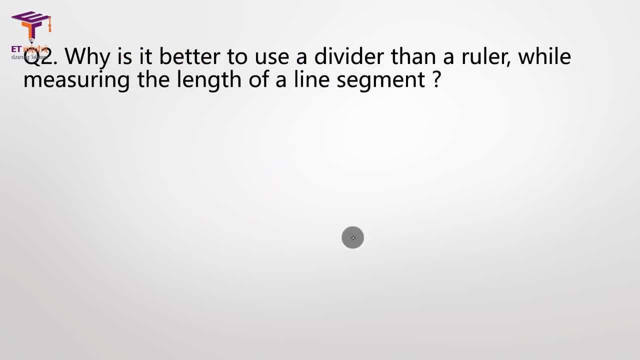 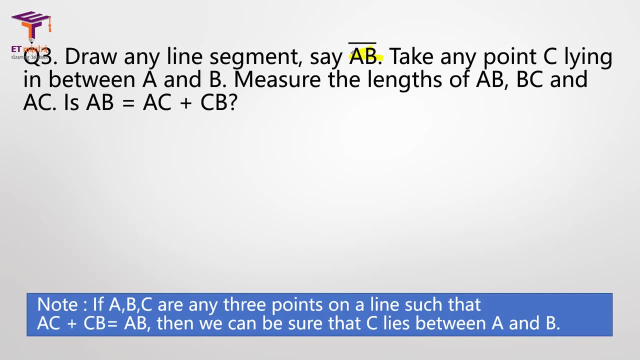 i want to go to the next slide. i will simply swipe, then swipe see, you can see. these notes are also available and because i already have this highlighter, i can use this highlighter to highlight some text, or i can select a pen to start solving this here. so, like, let me write, then you can start solving this question here. 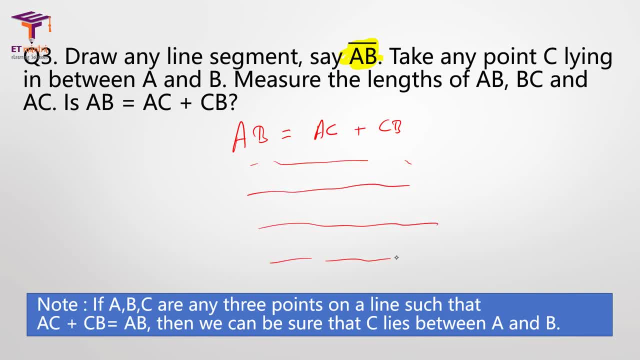 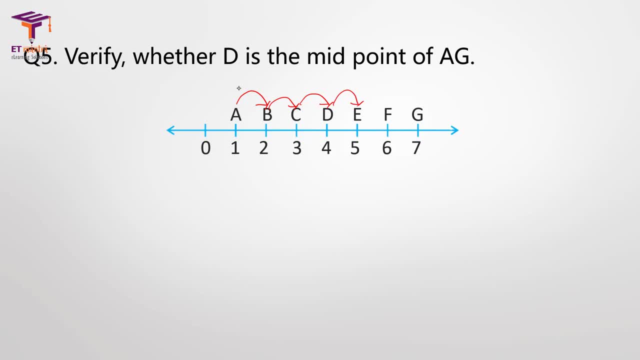 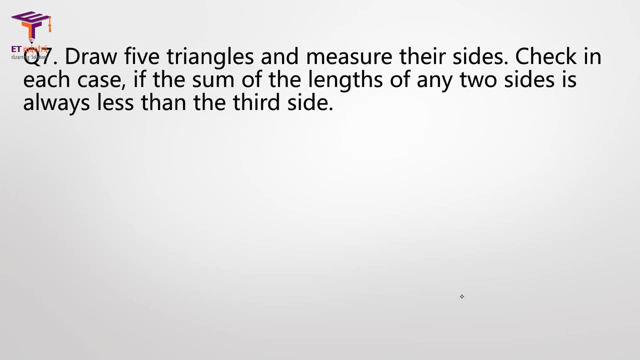 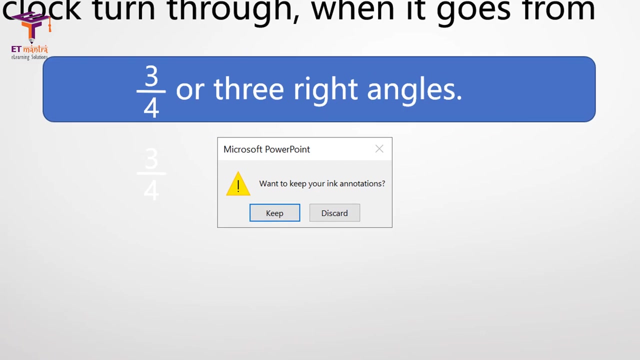 and once you are done, you can simply go to the next slide by swiping, so this way you can teach everything. once you complete this presentation, stop the slideshow. it will ask you whether you want to keep the annotations or not, and this time you know that you have to keep the annotations once you. 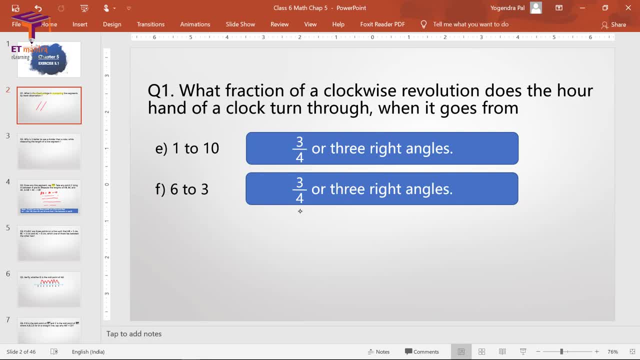 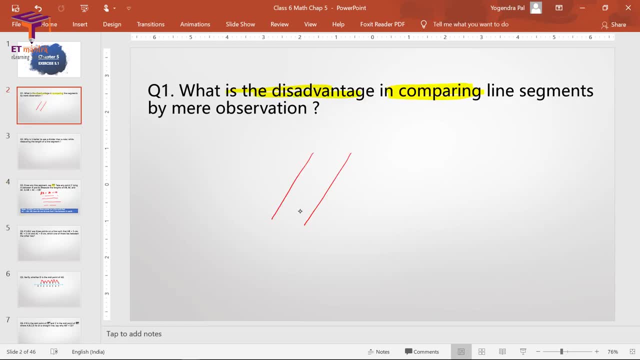 click on this with the text, which was already there, you have these handwritten notes also, so this way you can combine the text with the annotations. so this way you can combine the text with your handwritten things during teaching and finally share this file to convert this file into pdf and share it with your students. so now i believe you know how to write on.